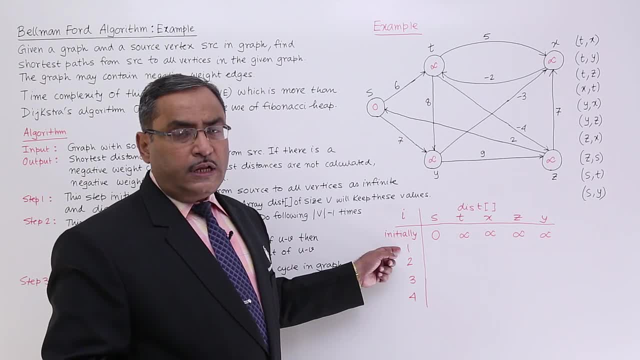 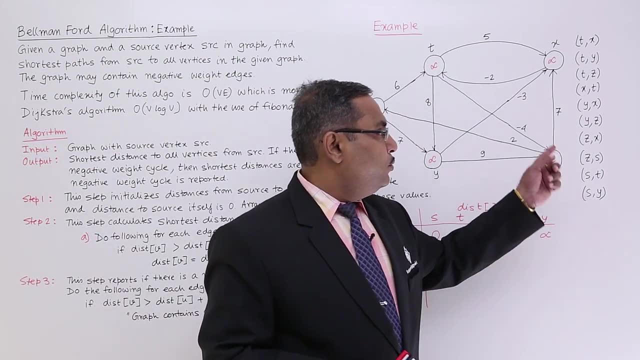 one in the graph. So now I shall go for step number 1, that is, the loop number 1.. So now, before going for the first time looping, this is the list of edges we have written. it is a simple list. there is no particular order in which I am. 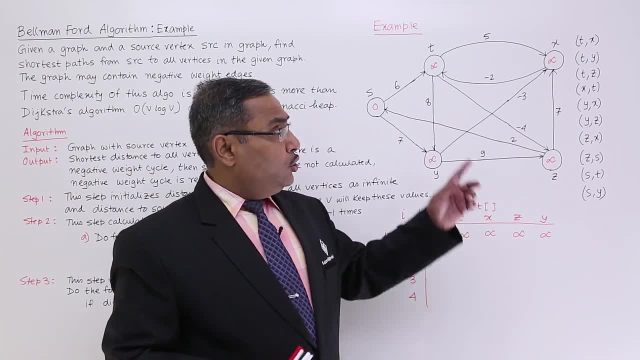 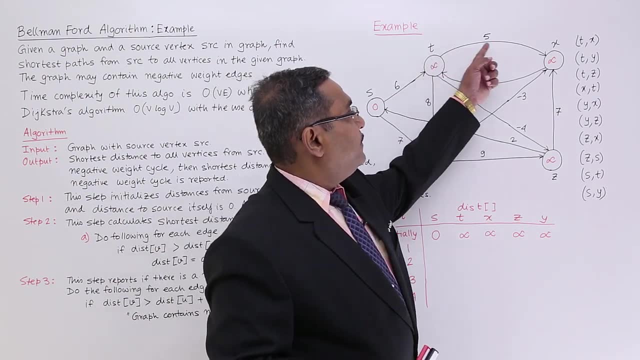 supposed to write them. I could have written them in other order also, So we shall trace this particular edges in this particular order. So t x means we are considering this particular edge in this way. we have written this one in an arbitrary order. Now we are going for. 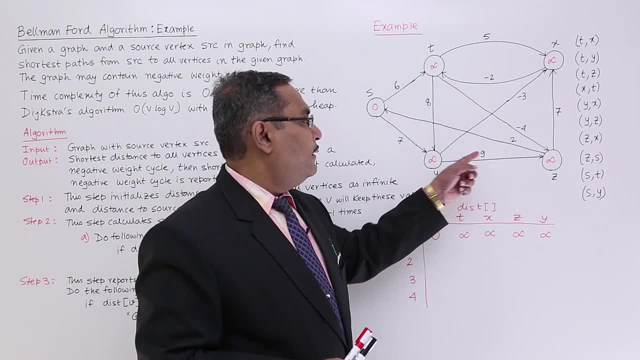 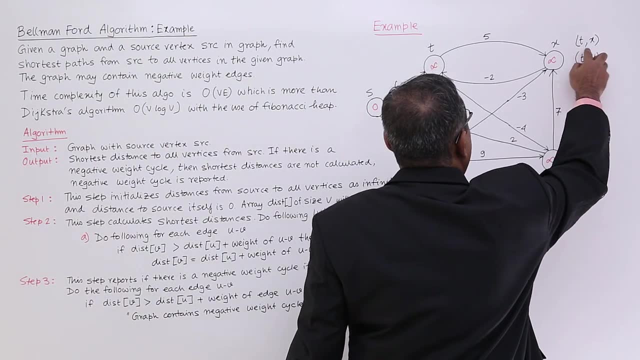 this step number 1.. So I have written this 0 and infinite values. so I have written this one. I am going for step number 1.. Now it is counting this t x. So t x means so we shall go for infinity plus phi. that. 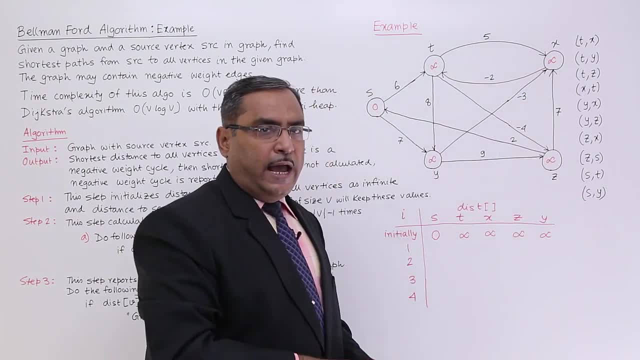 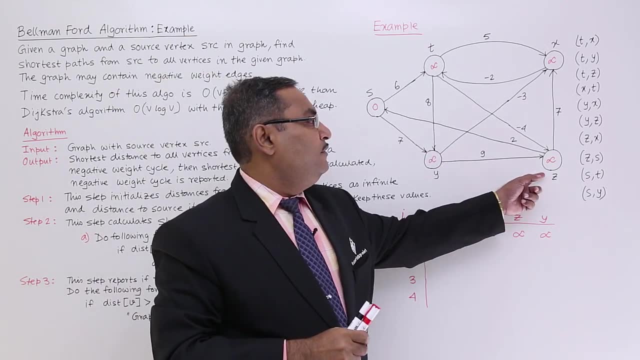 is infinity, so it requires no update. Actually, if you consider in this way all these edges which are not coming out from this s, all the values are infinite, so infinite plus is respective width, it will become infinite, so that will be no updated. 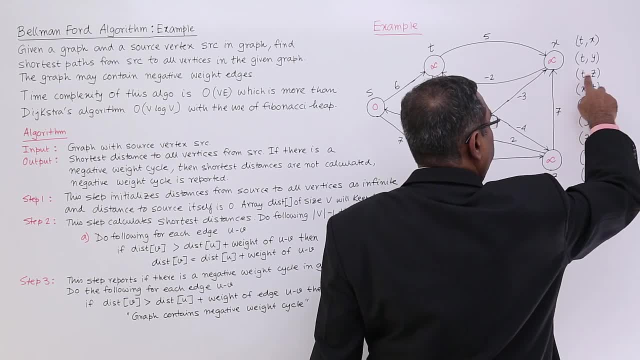 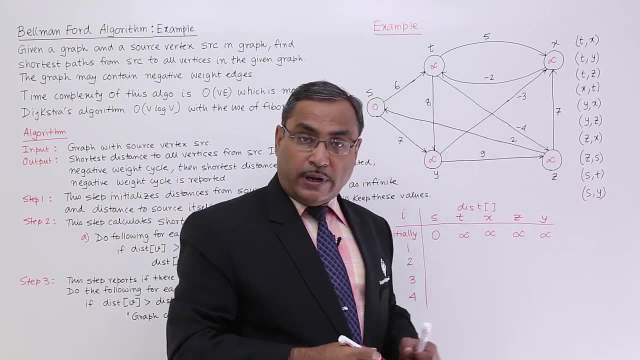 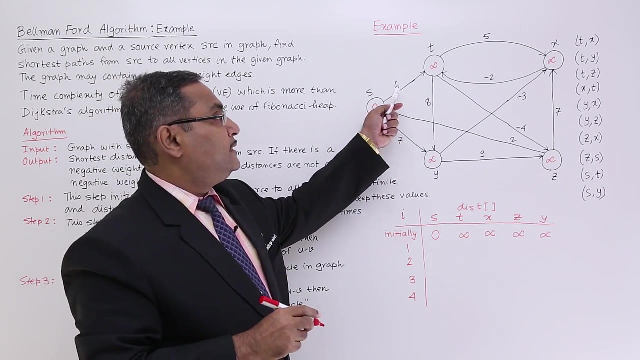 So in case of initially, I would need not to consider this one. if you consider also, the narrative will not have any update in the distance value. So I should consider only s, t and s? y, because s is having the respective distance value is 0. So 0 plus 6 will be getting 6 here for t. So I 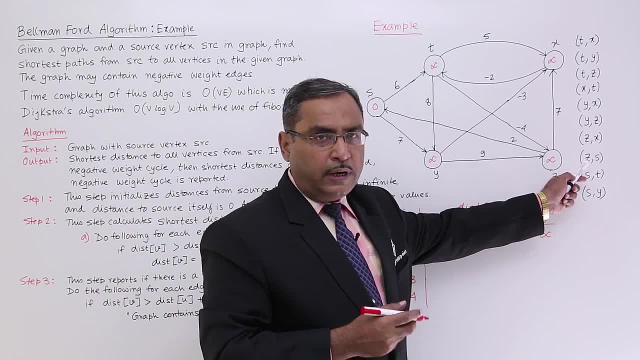 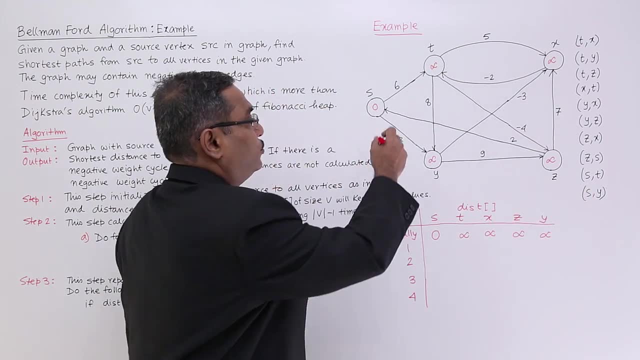 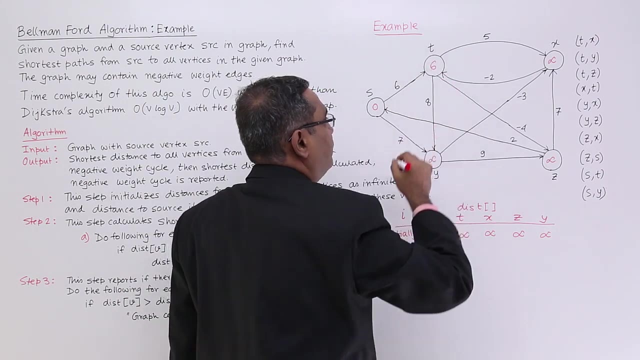 am considering this particular age. I considered already all of them, but there was no update in the respective array dist. So I am considering s of t at first. So s of t, so now s to t, rather. So 0 plus 6, I am getting here 6, because 6 is lesser than infinite, So that 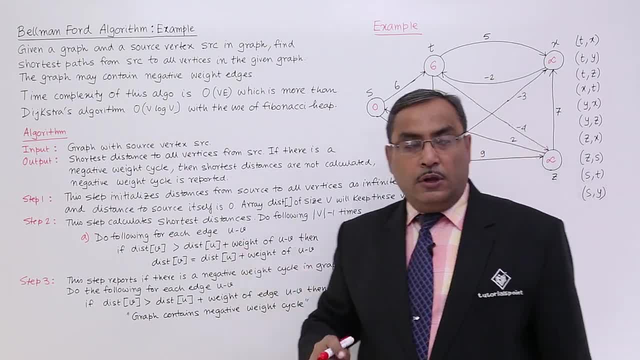 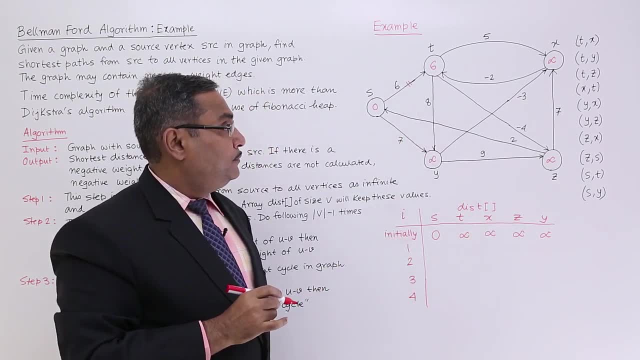 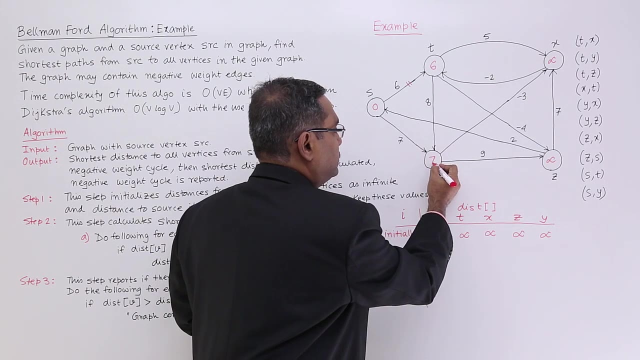 is why this particular step. So 6 is less than infinity, So that is why 6 has been put. So that means I have considered this particular age. So now we are having this 7.. So 0 plus 7 is 7.. 7 is lesser than infinity, So I am putting this 7 here. So that means 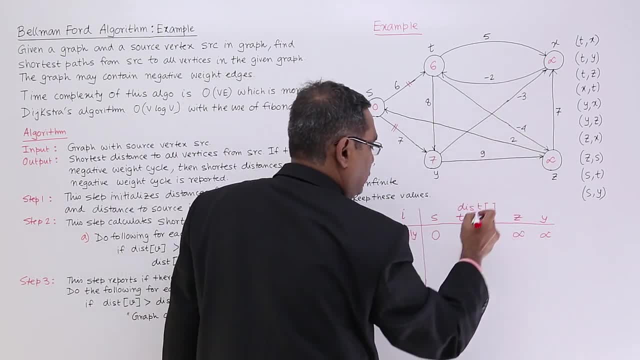 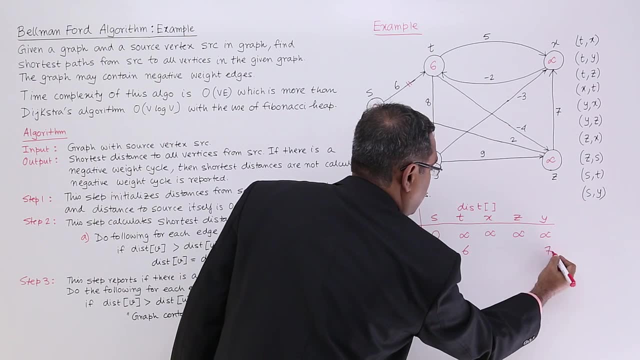 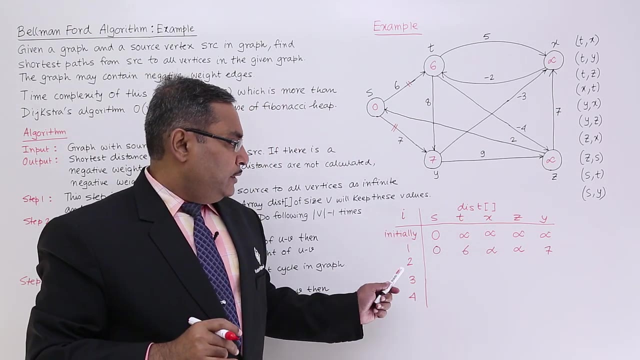 I have considered this particular age. So now, after this particular update, I am having this value 0, obviously previously, and t will have the value 6 and y will be have the value 7 and rest will have the value infinity. So these two edges I have selected. Now we are going for iteration. 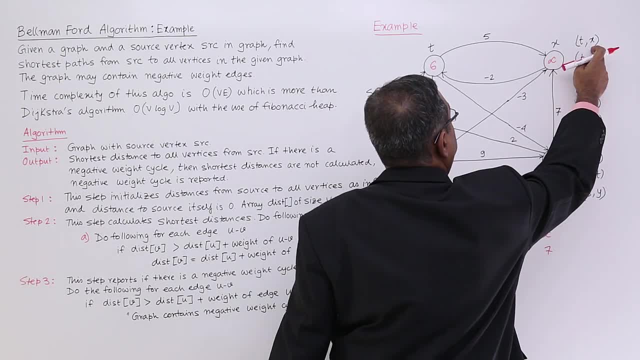 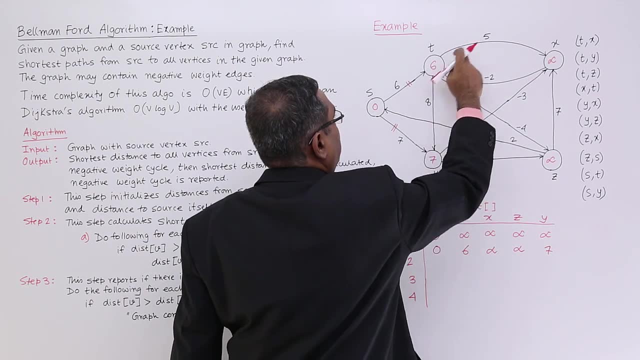 number 2.. In the iteration number 2, we shall consider this: t, x So t plus x So t. x means this edge, So this particular distance plus weight, So that is 11.. 11 is lesser than. 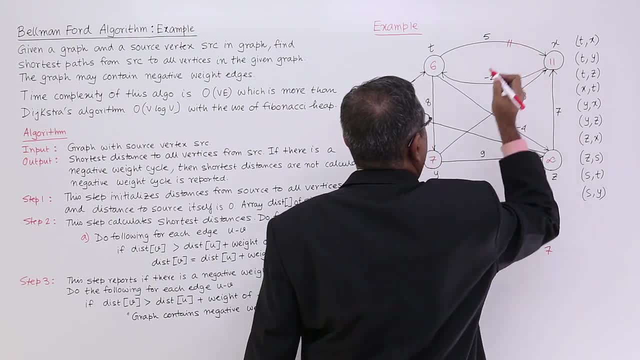 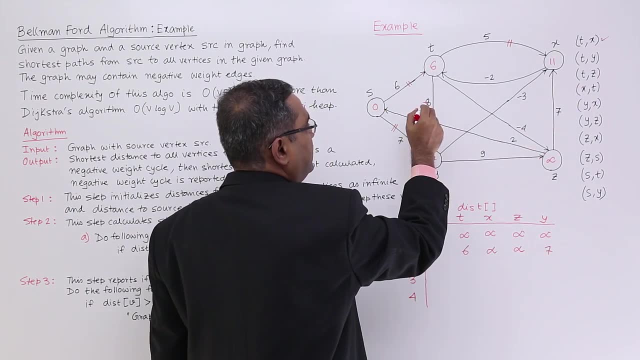 this, So 11 will be coming down here. So I am considering this particular edge. Now we are going for t y, So going for t y, So t y means this one, So 6 plus 8, that is. 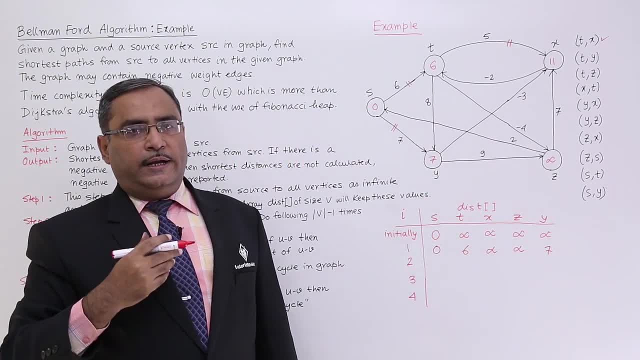 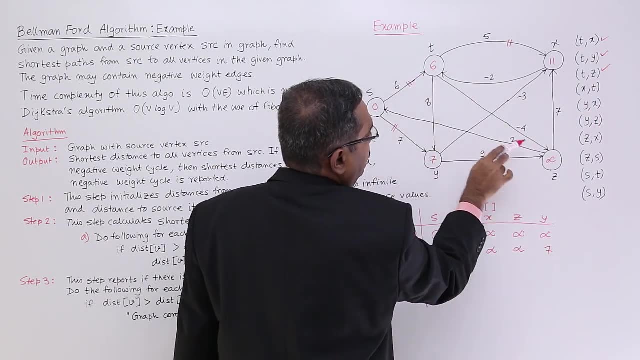 14.. 14 is greater than 7. So it does not require any update. We are going for t z now. We are going for t z. So t z, t z means this one. So 6 minus 4, that is 2.. So 2 is lesser. 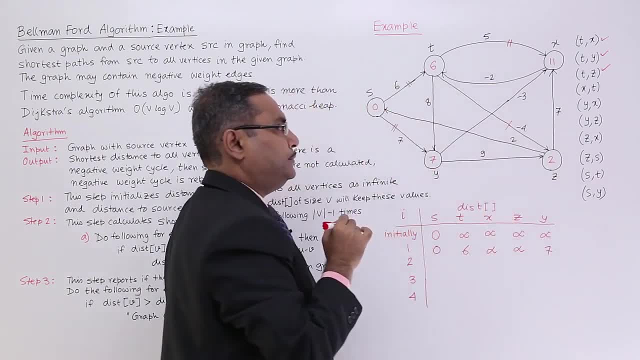 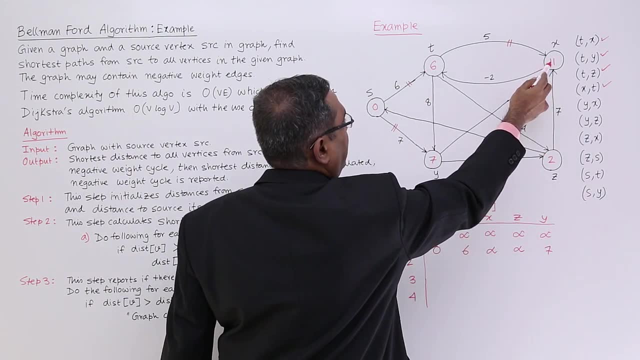 than this value. So I am putting this one. So I am considering this particular edge. I am considering this particular edge. So now I am going for x t. So x t means this particular edge. I am going for x t. So this is my 11 and this is my minus 2.. So that 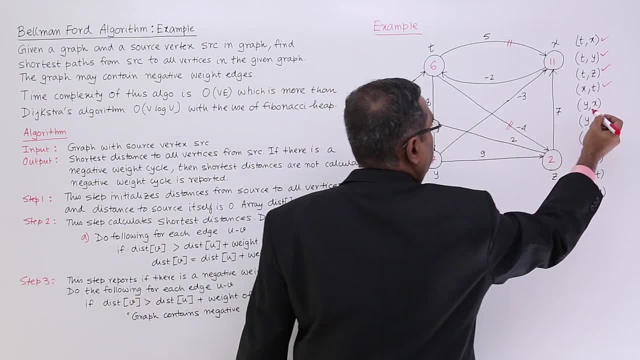 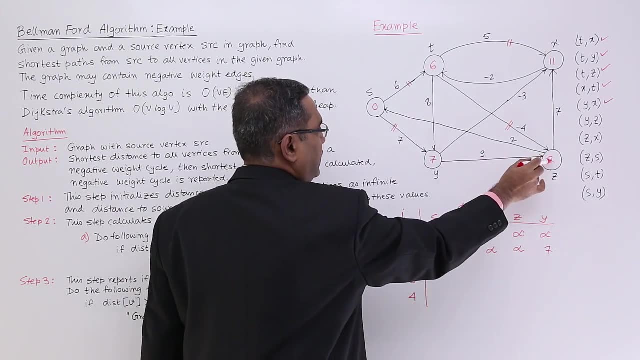 means 9.. So 9 is greater than 6.. So there will be no update. Now. I shall go for y z, I shall go for y z. So 7 is there, 9 is there. So that is 16 greater than 2. So no update. 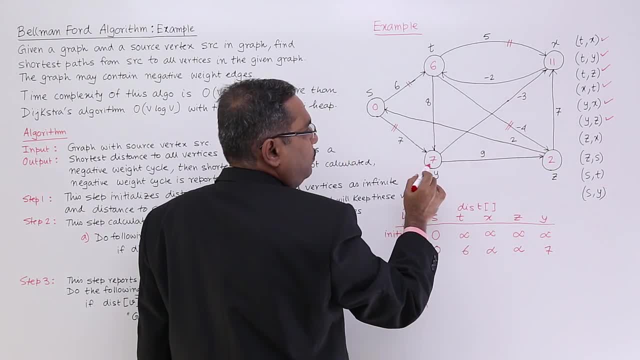 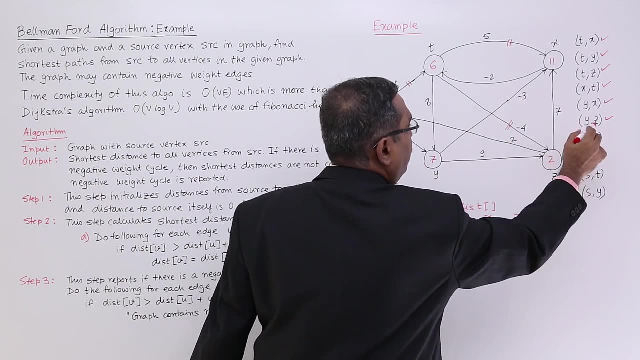 We shall go for y z, So this is my y. So I think I have gone for this Y z, So y x is this one. Okay, Let me go for y x at first. Okay, Y x means this one. 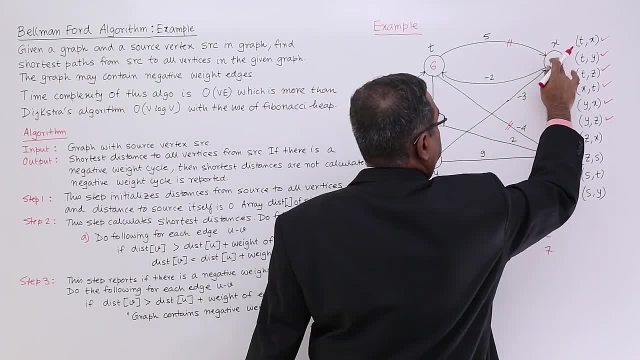 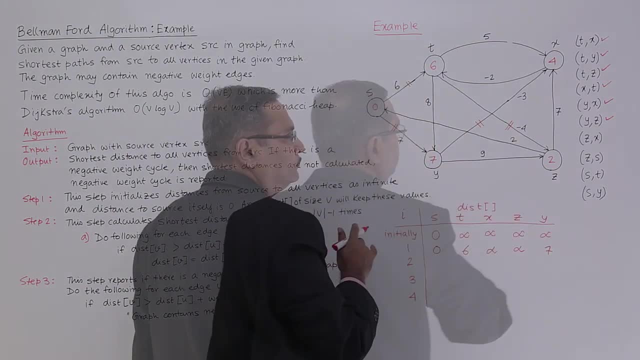 So 7 minus 3. So that is 4.. So 4 is lesser than this, So I am taking this one. So this edge I am not considering. I am considering this particular edge now. Okay, Now let us. 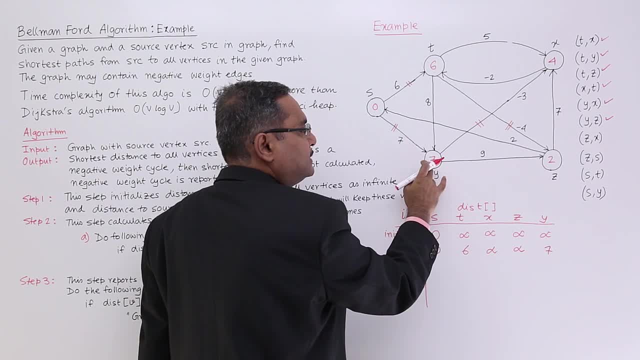 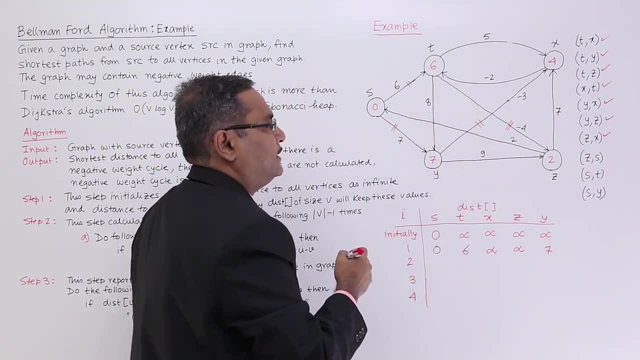 go for y z, So y z. we did this one, So 7 plus 9.. That is my 16.. 16 is greater than this, So there will be no update. Go for z x. So now, if you go for z x, you will get. 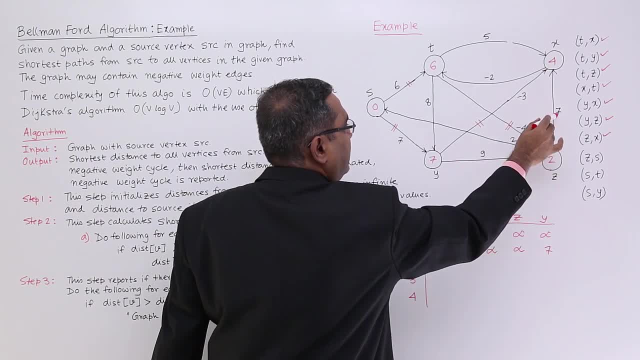 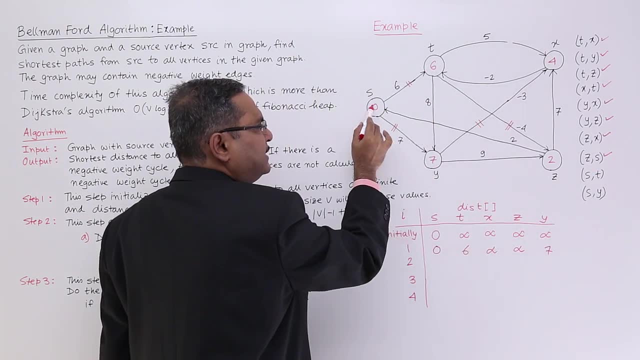 z x. So that is the edge. So 2 plus 7. So that is 9 greater than 4. Need not to have any update. So z s. So for z s z s is 0. So it cannot be. it should not be. 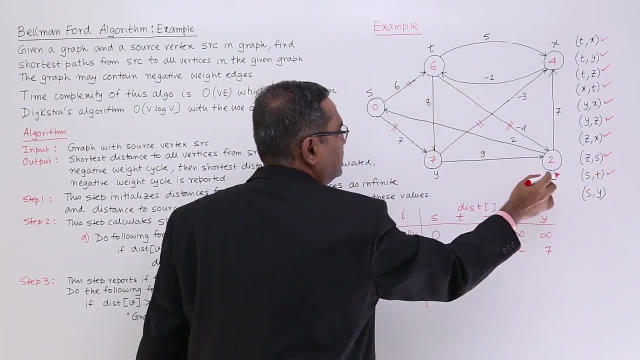 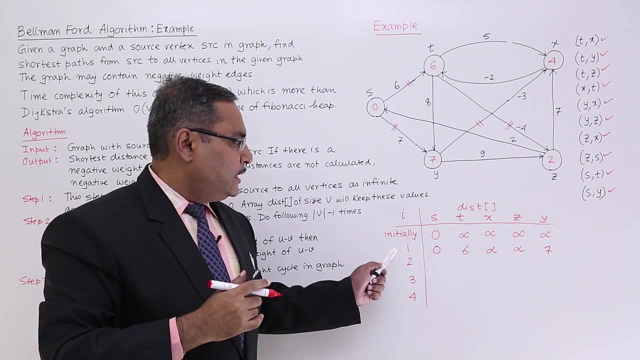 considered, So it is already. So I should not consider this z s And this is my 0. So I should not consider them. So they have already been considered. So in this way, for the iteration number 1, I have done this. Now for iteration number 2, my updates are: 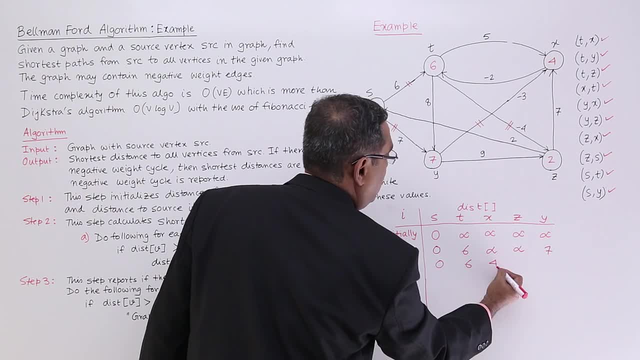 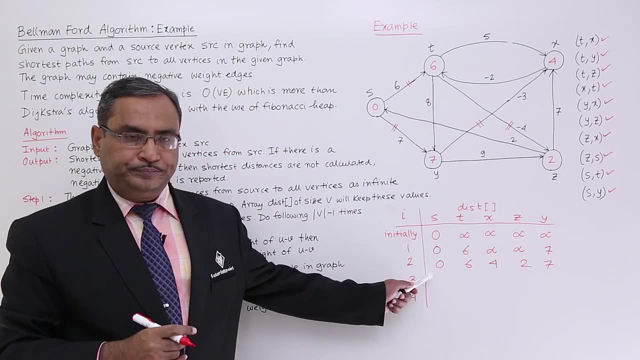 0. And then 6.. So x has got 4., Z has got 2. And y is still remaining with 7.. So in this way I have got it. Now I shall go for iteration number 3.. Okay, So t, x, t x means. 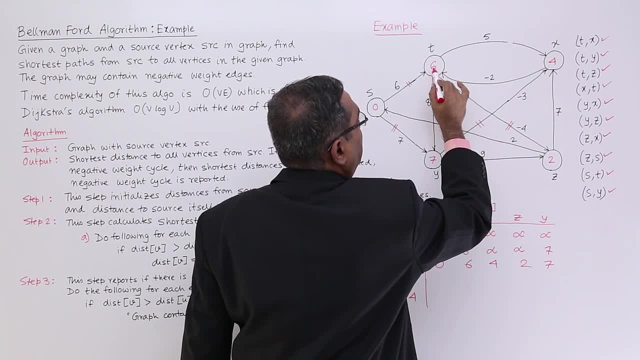 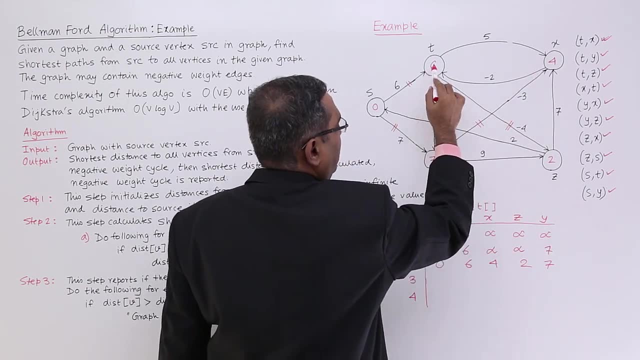 this one. t x means this one. So 6 plus 5, 11.. Sorry, it is not, should not be, should not have any effect. So t y, t y means this one: 8 plus 6, no effect. 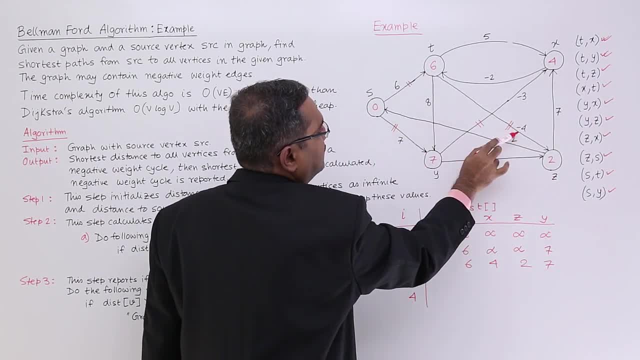 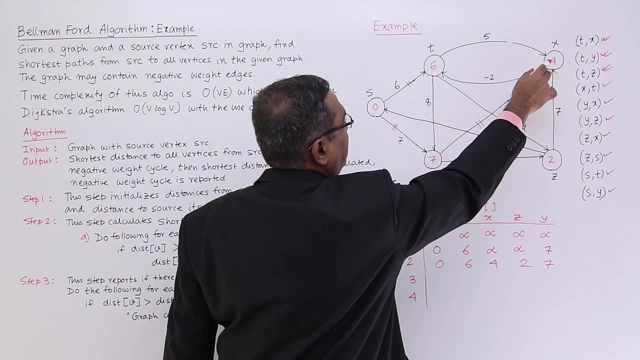 We are going for t z, So t z means 6 minus 4 already taken. x t, x. t means which one? So I am going for this x And this is my t, So this is my minus 2.. See, this is my. 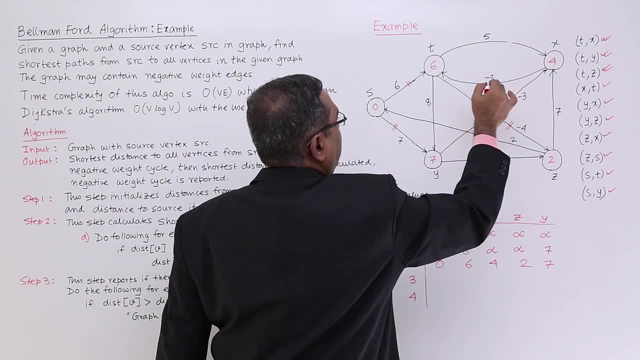 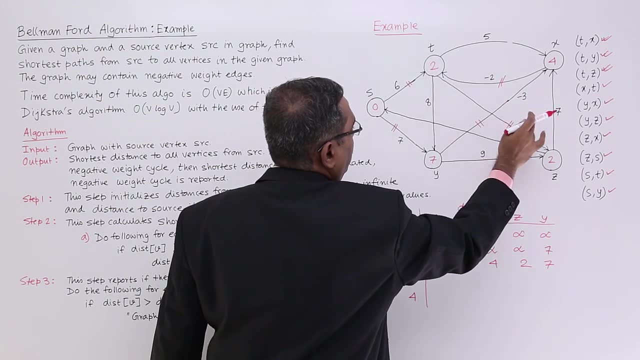 minus 2.. So 4 minus 2.. And that is my 2.. So 2 is lesser than this. So I am writing this one, this one. So this is I am taking. I am not taking this, I am not taking this. 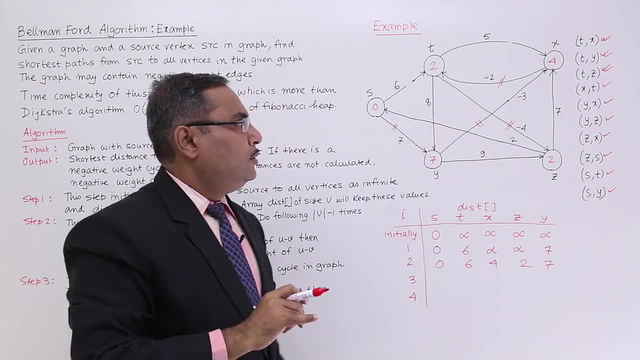 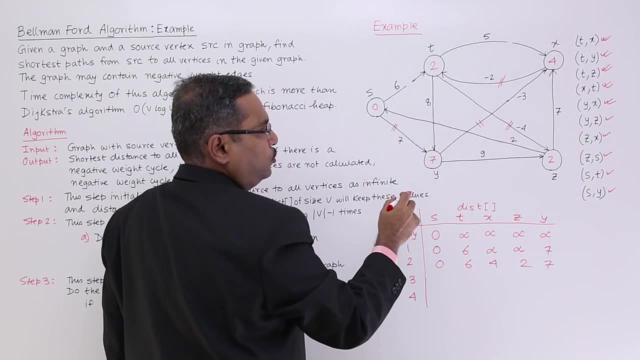 Because this is the shorter one. I should not take this one. Okay, Now we are going for so x t. we have done So. now I am remaining with this y z. So y z means this age, So 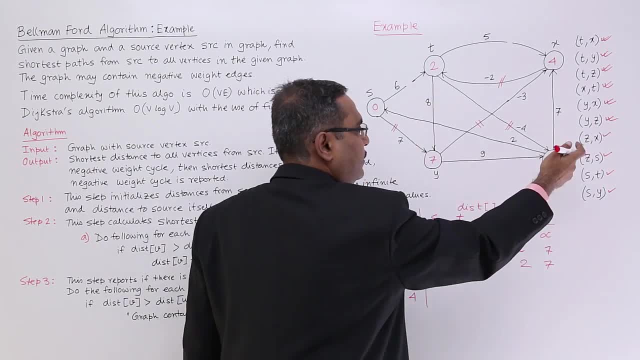 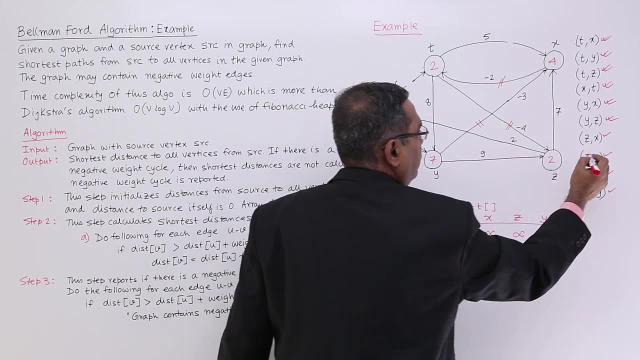 need not to be considered Because it is 7 plus 9.. In this way you can proceed: Z- x. We are going for z x, So z is this one. So 2 plus 7,, 9 greater than 4.. So it has. 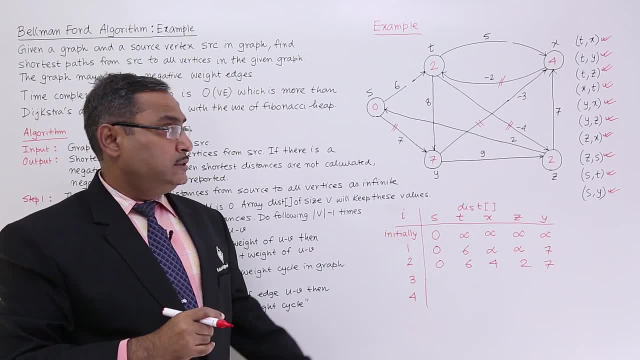 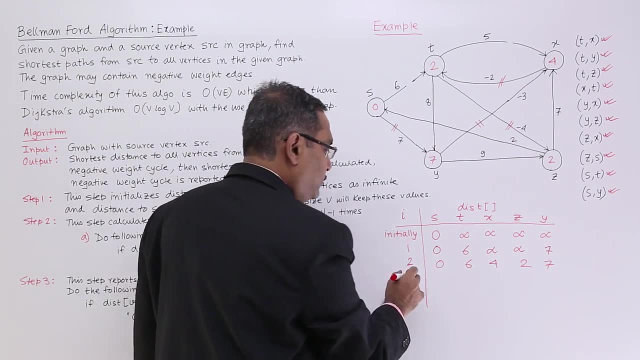 been considered already. There will be no updates there. S is 0. So it will be always have the minimum value there. Now we are going for iteration number 3.. So iteration number 3, then I am having one update here, So x will remain with. 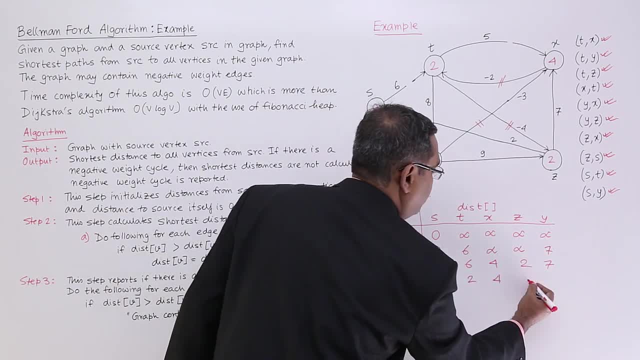 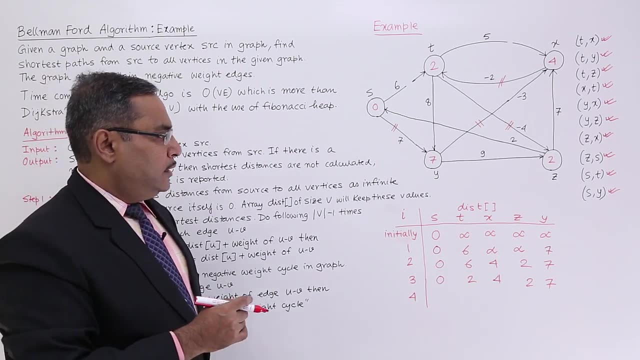 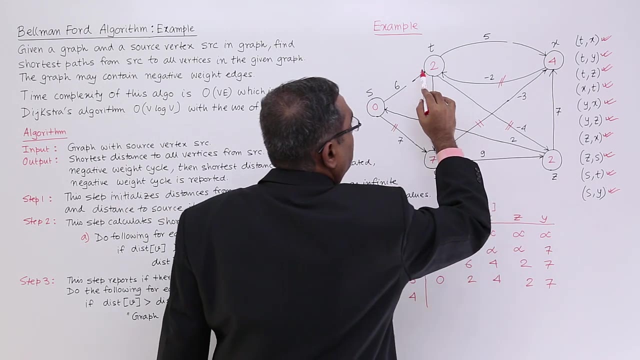 the value of 4, z with 2 and y with 7.. Now let me go for the last one, that is 4, fourth iteration. So go for t x. So t x, no effect. Then go for t y. t y means this one. 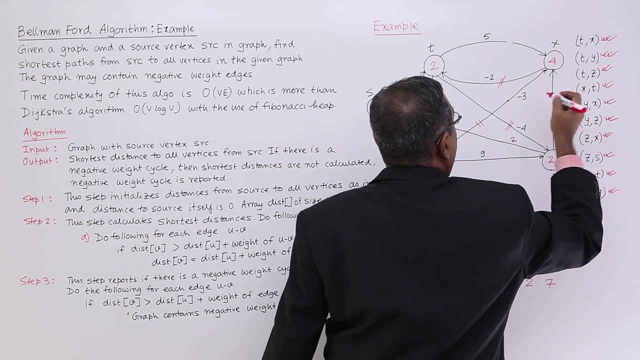 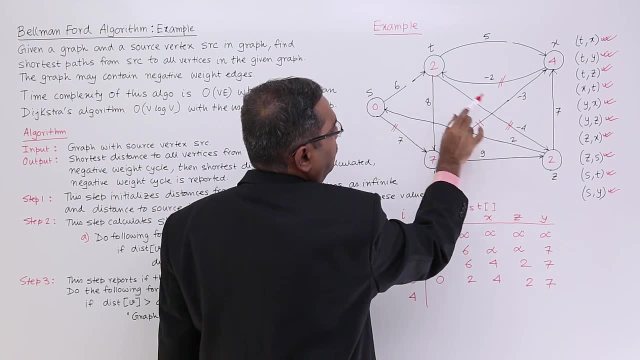 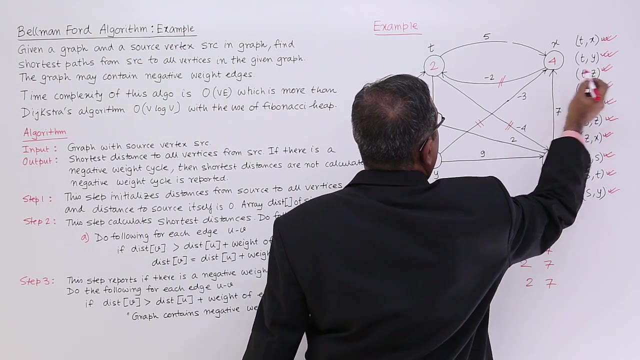 So 8 plus 2, 10, no effect. Go for t z, So 2.. So that is my 2 and that is the minus 4.. So it is already considered here. Now going for t z, we are having this one. 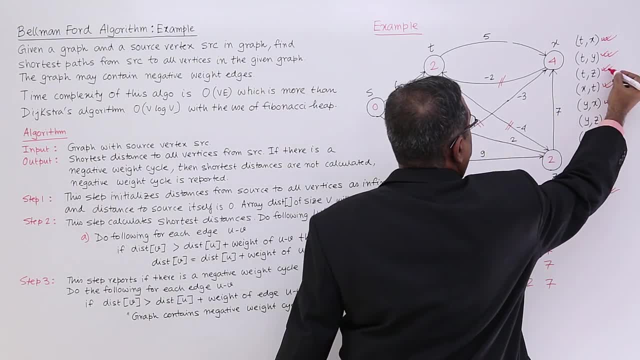 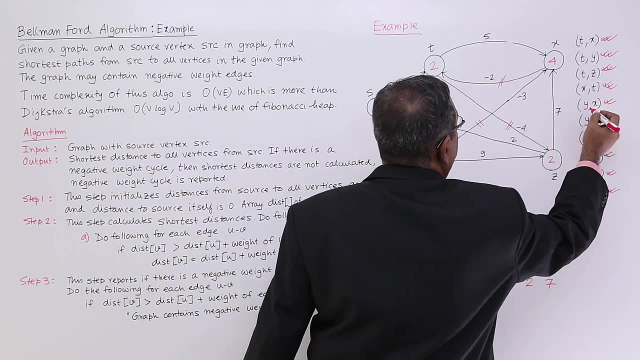 So t z. this particular age has already been considered. t z. Now go for x t. So x t means this one, It is already considered. Now go for y x. So this is my y, this is my x. 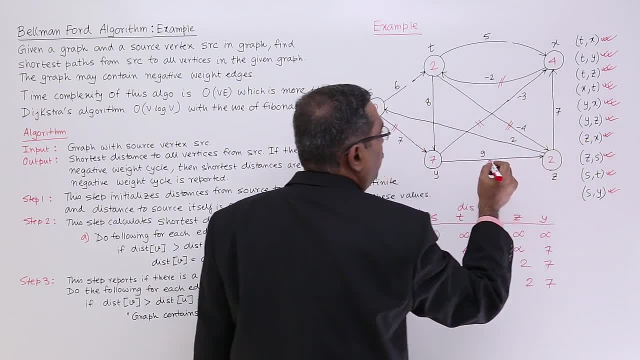 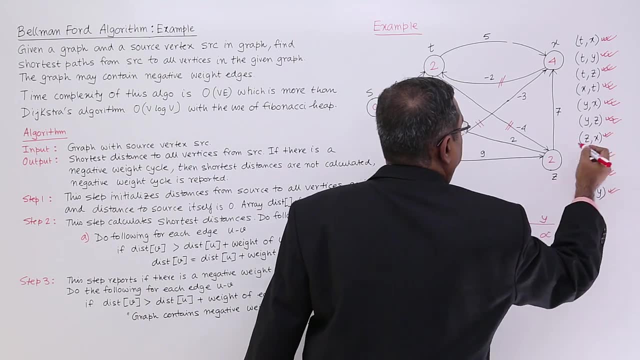 So this particular age has been considered already. So go for y z. So that is my y and that is my z. So 7 plus 9 cannot happen. Go for x z. x z means I am having this one, x z means 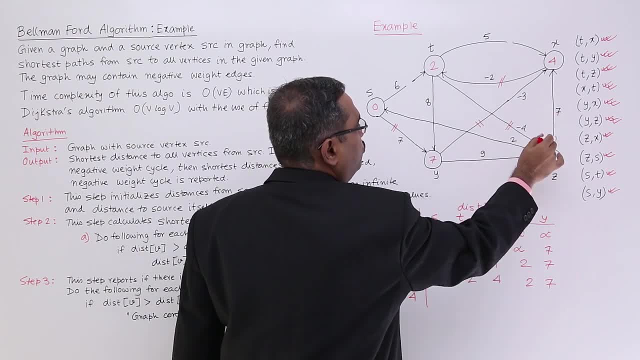 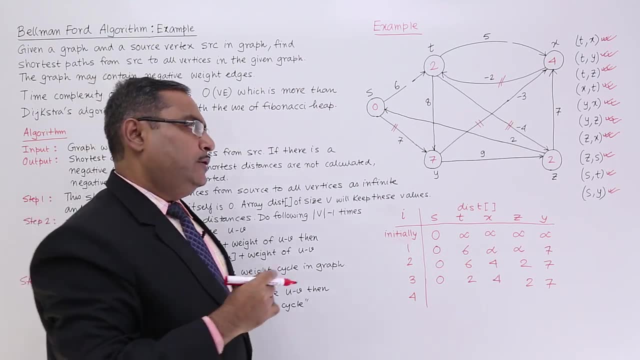 this one. Now go for z x. z x means this one, So 2 plus 7, 9 is greater than this. So z s, s, t and s y will not have any updates because that is involved with the s and s is. 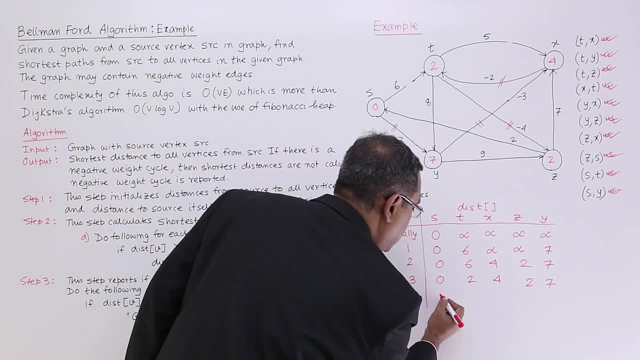 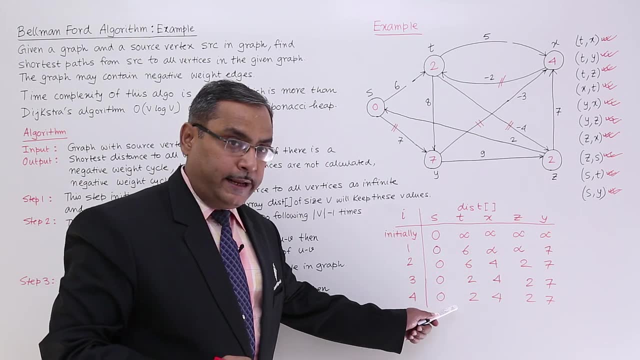 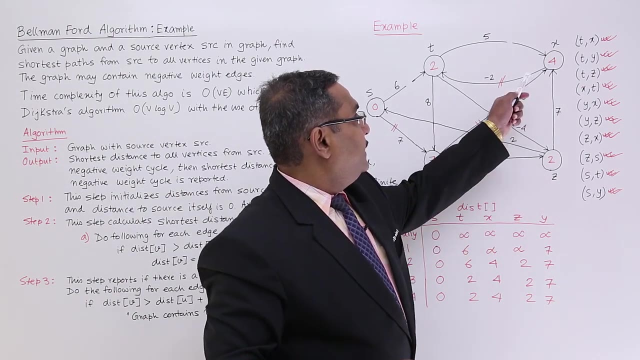 having the minimum dist already. So this particular dist array will have no updates afterwards. So in this way the things are taking shape. So now you see, we are having this particular age, This particular age, this particular age and this particular age, So we are having 5. 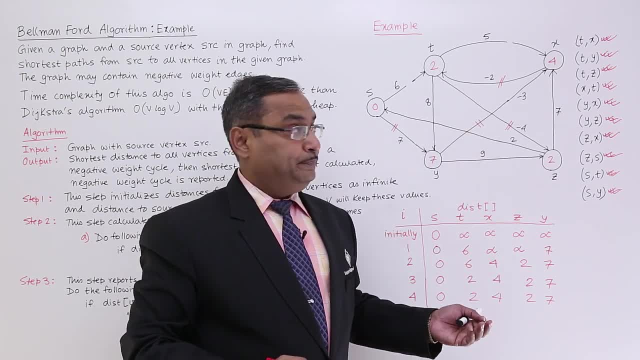 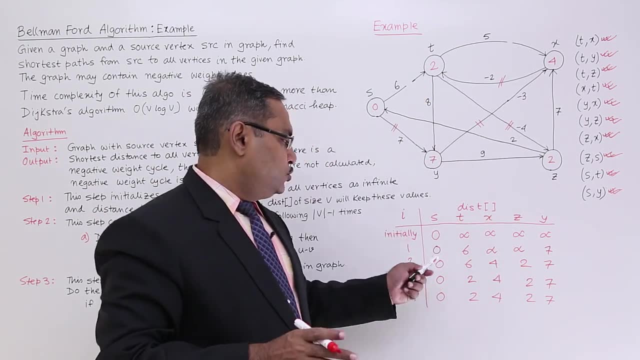 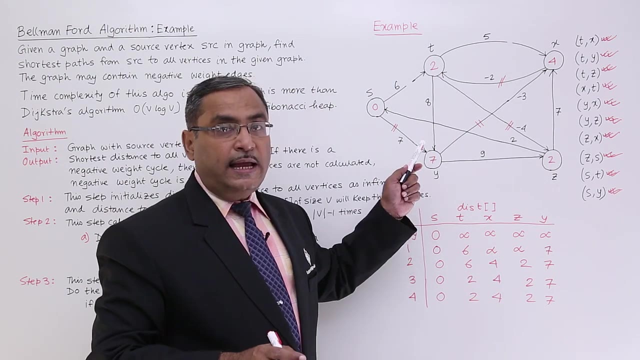 vertices, We are having 4 edges to connect them From the source vertex. in this way I found out the shortest path to all other vertices. So that is my dist array final status and that is the final graph condition. So in this way the algorithm is executing. So now, here it is. 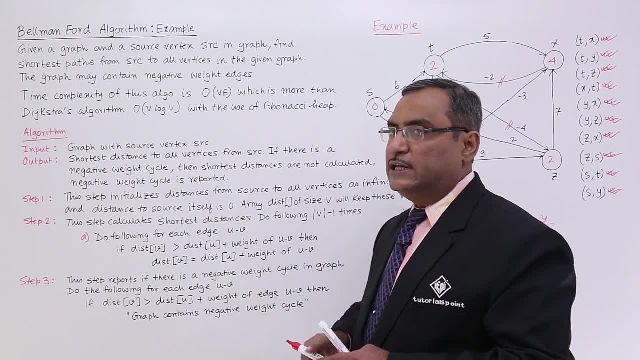 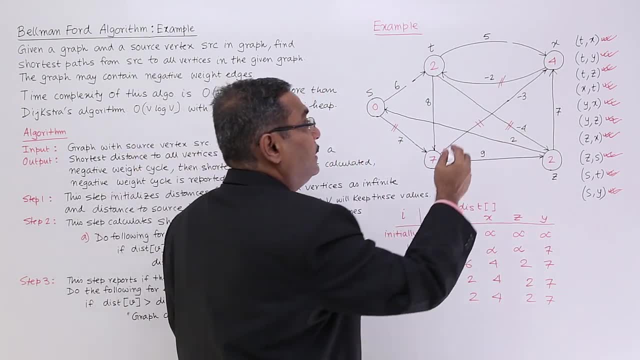 asking for any weight cycle: negative weight cycle, negative weight cycle. negative weight cycle is present or not? Yes, that is, the negative weight cycle is there. That is the negative weight cycle is there, and that means this particular negative weight cycle indicates. 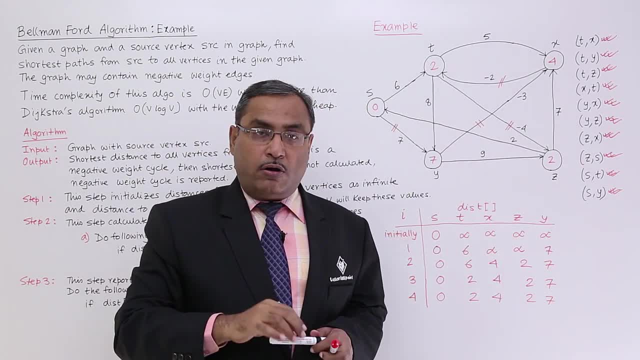 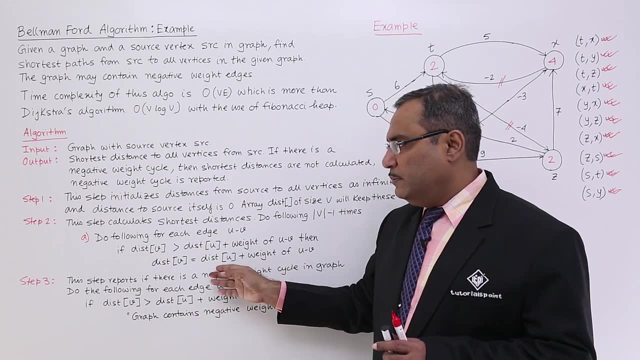 that we can reduce these distances later on for the multiple time application of the negative weight cycle. So that is why I am not going to do any updates, because it has been mentioned that just report that it is having negative weight cycle. So graph contains negative. 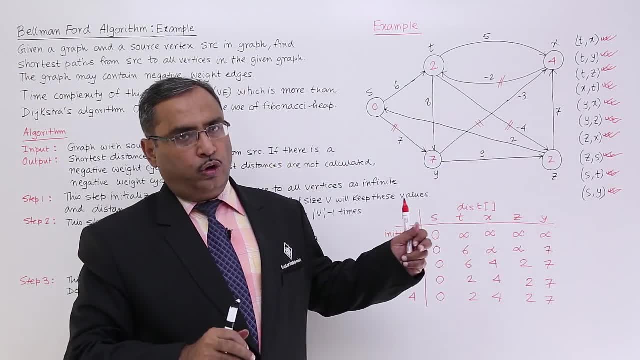 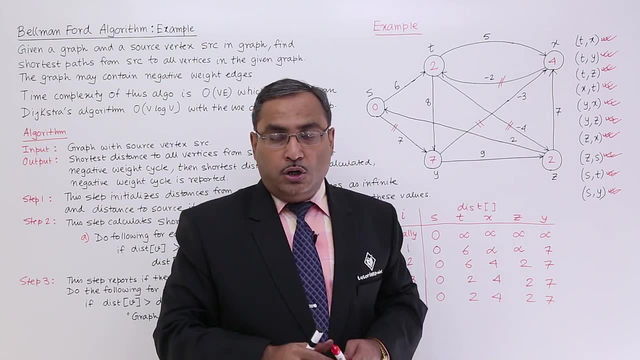 weight cycle. So that reporting, that notification, that reporting, that reporting, that reporting this algorithm will make at the end, because that is a negative weight cycle, So that is a cycle with a negative weight. So in this way, the Bellman-Ford- how does a Bellman-Ford algorithm?